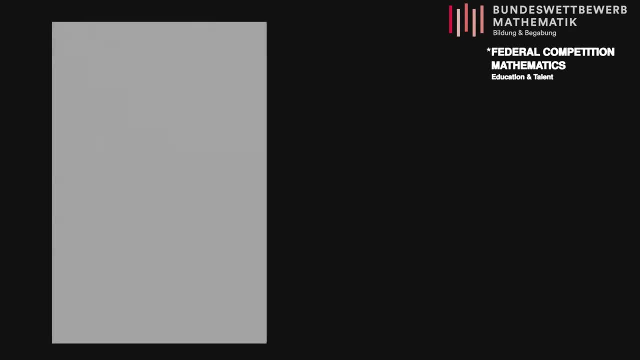 Let me introduce you to the Bundeswettbewerb Mathematik, one of the biggest German math competitions for school students. The first round is three months long and participants are asked to solve three out of four problems at home. Students managing to do so face four harder problems in the 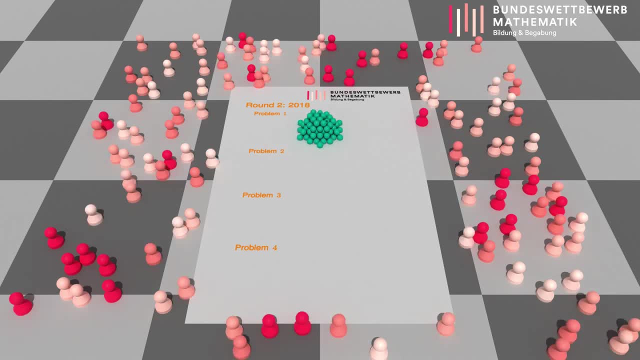 second round, but this time they only have two months and need to solve every problem in order to progress. They are not only allowed, but actually encouraged to study math literature while problem solving, And yet despite the abundance of time and resources available. 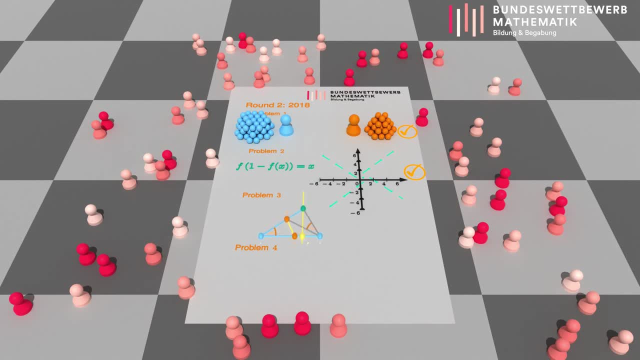 a lot of students unfortunately fail to solve every problem. In the year 2018, only 22% of the competing students actually managed to pass the second round. This makes it apparent that these problems are genuinely hard. In this video, I am going to discuss the 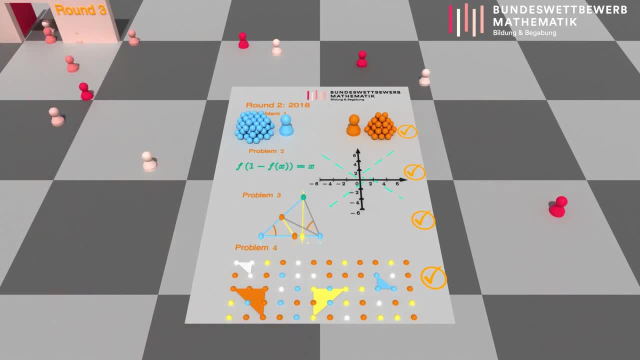 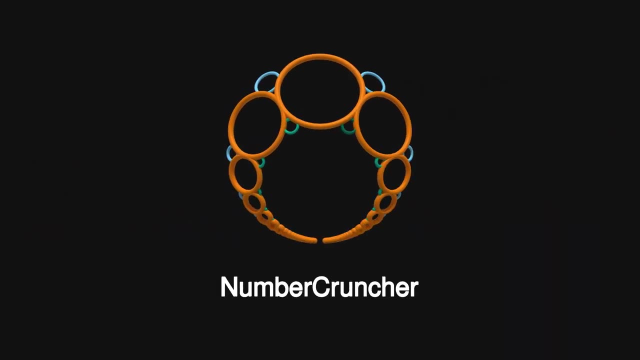 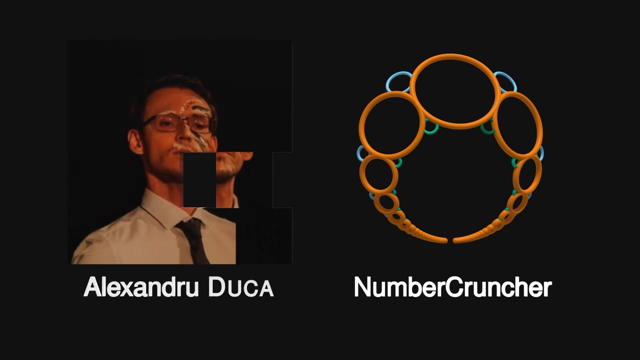 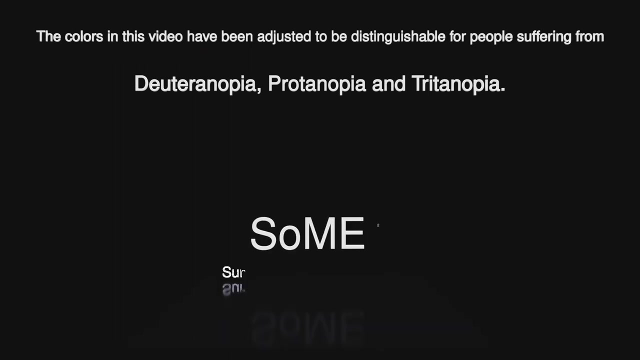 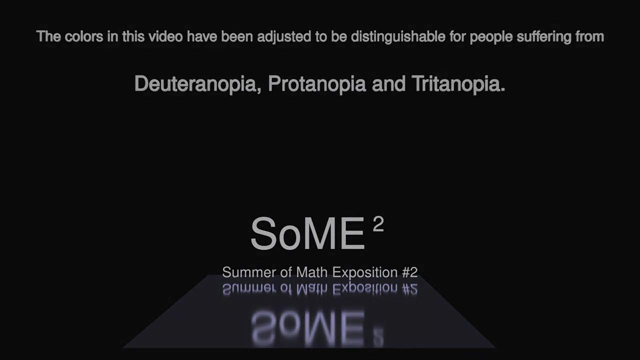 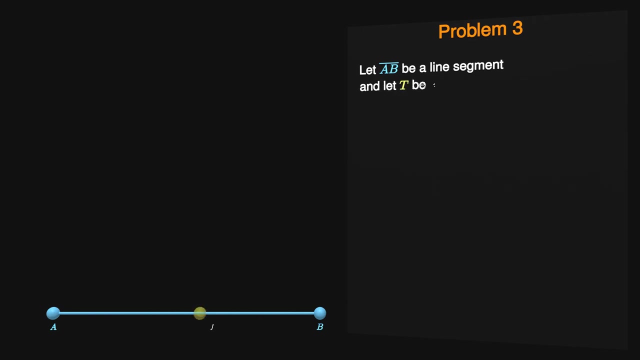 geometry problem from that year and show you a technique that turns it into a small exercise. Until then, thanks for watching and don't forget to subscribe. Here's the problem. Let AB be a line segment and let T be a point on it that is closer to B than to A. 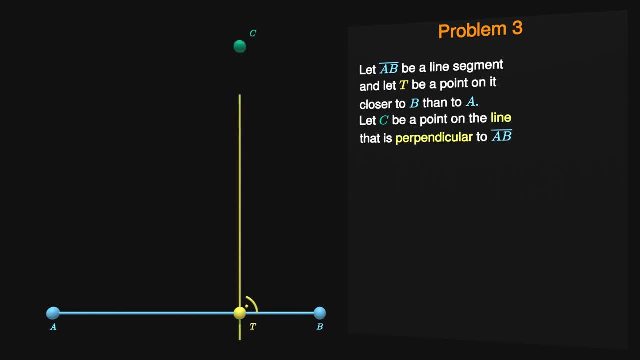 Let C be a point on the line that is perpendicular to AB and that goes through T. First, show that there exists exactly one point D on the line segment AC, such that the angles CBD and BAC are the same. Second, show that the line perpendicular to AC and going through D intersects the line. 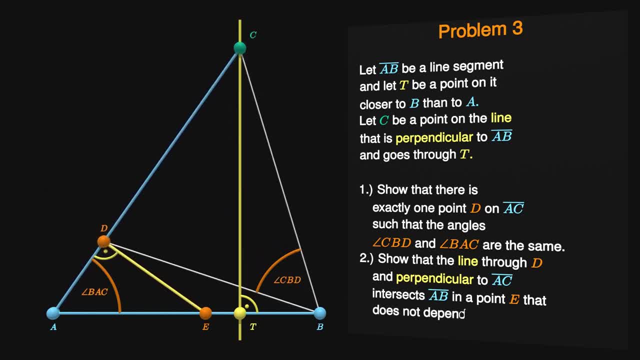 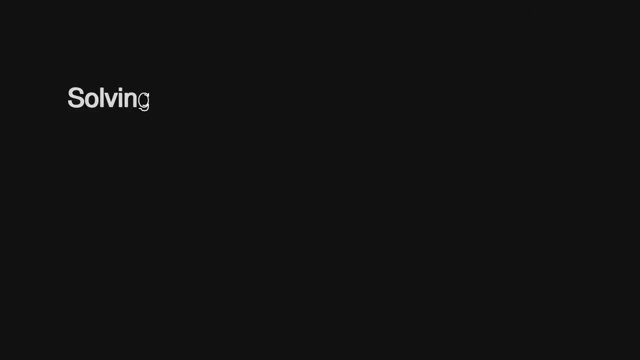 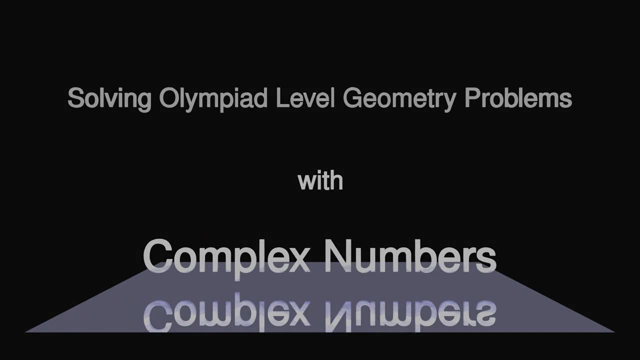 segment AB in a point E that does not depend on the choice of C. I am going to reveal the solution to this geometry problem by the end of this video, but first I need to introduce you to our main problem solving tool: complex numbers. 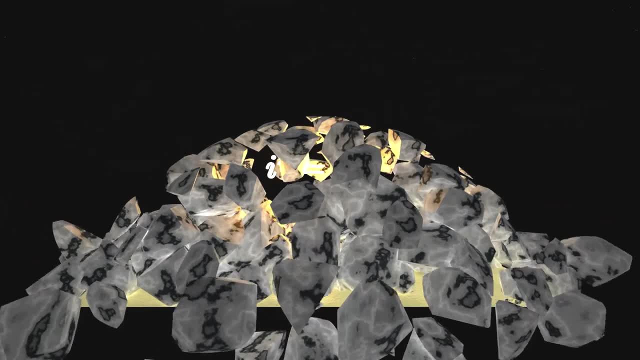 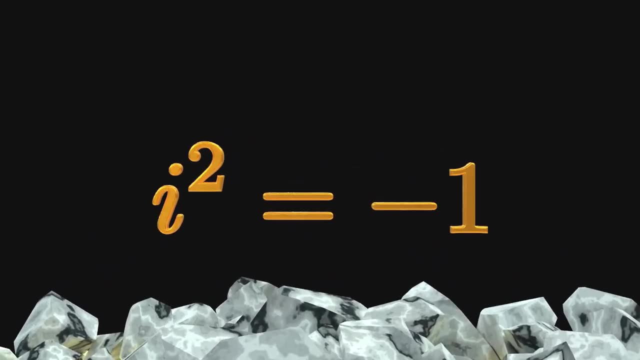 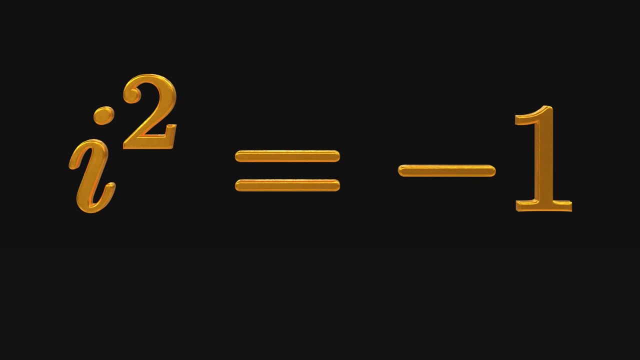 Let the number i be defined by the property that its square is minus one. Notice that it's not a real number, since the square of a real number cannot be negative. i is called imaginary. for this reason, While performing any calculations, we are going to treat i like a constant, while keeping 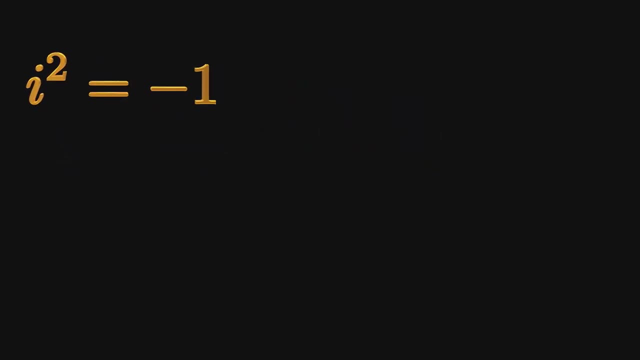 in mind that we can exchange, i squared for minus one. A complex number is a number of the form where a and b are real numbers. We refer to a as the real part and to b as the imaginary part, Two specific complex numbers. 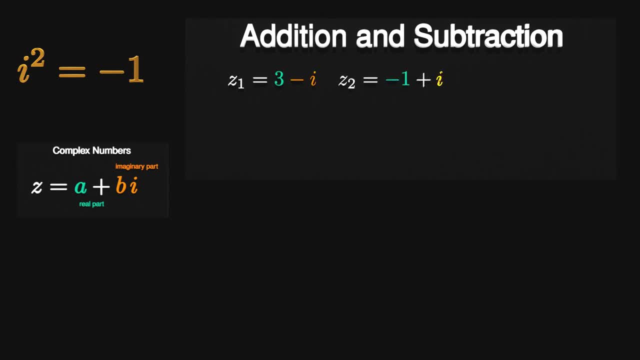 The first one has the real part 3 and the imaginary part minus one, while the second one has the real part minus one and the imaginary part one. Adding and subtracting these numbers is easy, as long as you remember to treat i like a. 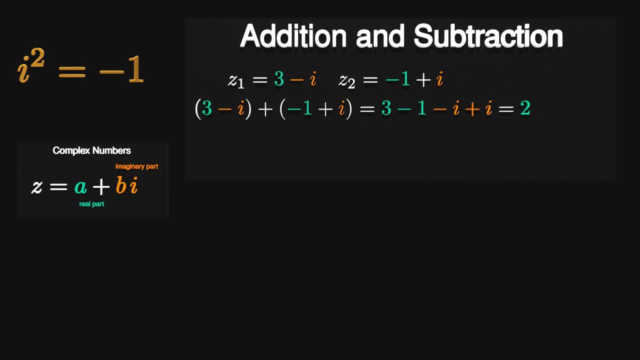 constant. Multiplication is just as easy, but this time you also need to remember that you can exchange. i squared for minus one. The trick when it comes to division is that you have to remember that the real part of division is to expand the fraction with a divisor whose sign has been flipped in the 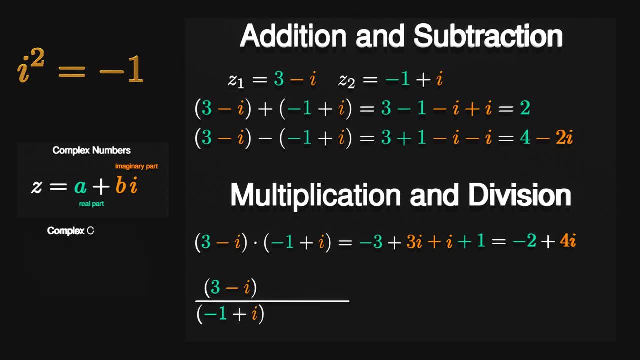 imaginary part. in this case, the term to expand with is minus one minus i. This operation might look the scariest, but it's actually just two parallel multiplications. Notice how i disappears in the divisor after multiplying. Please keep in mind that I chose this example specifically for this operation to work out. 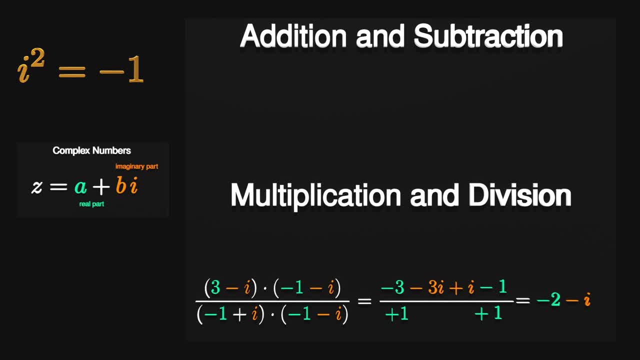 nicely. In general, dividing two complex numbers yields a messy result. Regarding the general case, it's useful to express these operations as formulas. Let's consider two general complex numbers- a plus b, i and c plus d. i, Where a, b, c and d are real numbers. 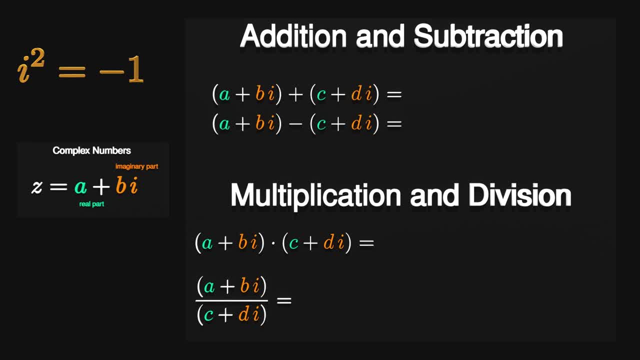 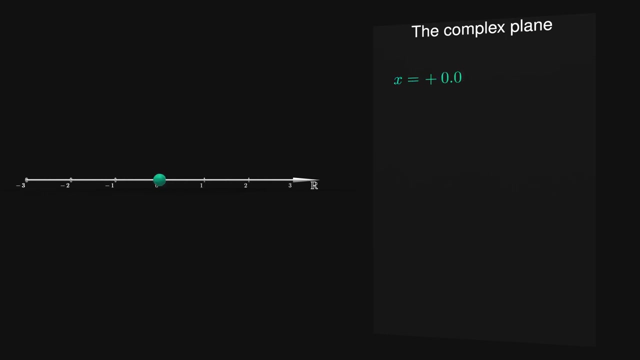 Pause and try to derive the following equations. In case of division c and d may not be both zero, since division by zero is undefined. Here are the results. Let's try it. Real numbers can be thought of as points on the number line, but i is not a real number. 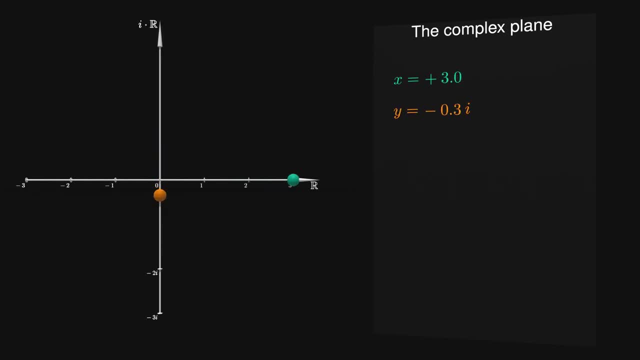 It lives on a line perpendicular to the number line, called the imaginary axis, and every multiple of i can be noted. There's a nuts and nuts problem. be found on it too. You can think of a complex number, for example 3 minus i as a point. 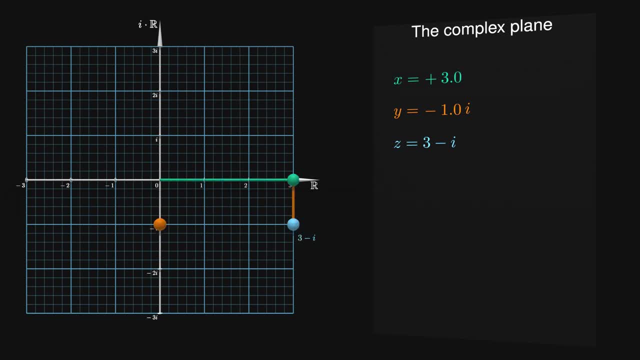 in this 2D space. The real part- in this case the number 3, tells you how far to walk along the real axis and its sign tells you in which direction. A positive real part means walking to the right, while a negative real part means walking to the left. The imaginary part in 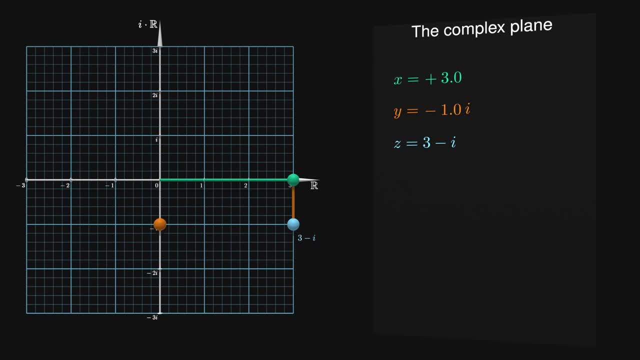 this case, the number minus 1, tells you how far to walk parallelly to the imaginary axis, and its sign tells you in which direction. A positive imaginary part means walking upward, while a negative imaginary part means walking downward. Notice how every point in this 2D space is associated with one and only one complex number. 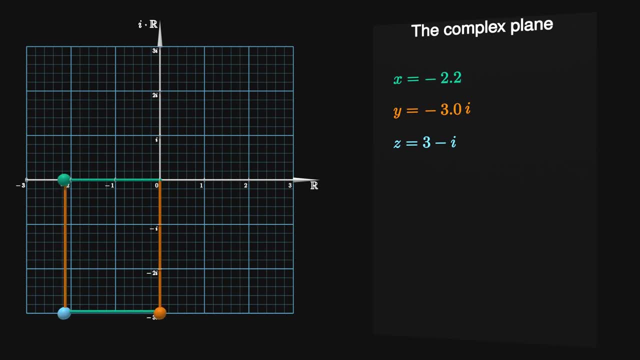 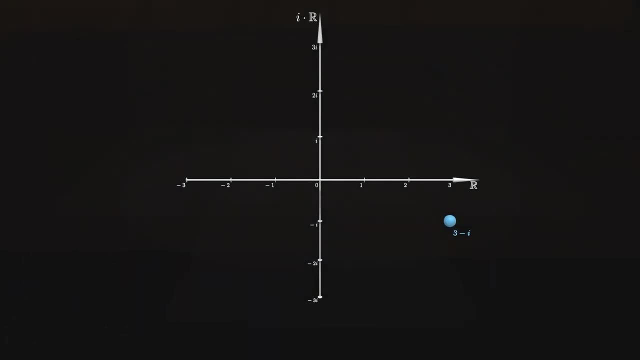 Likewise, every complex number is associated with one and only one point. For this reason, we call this 2D space the complex plane. If you think of our geometry problem as a theatrical performance, the complex plane is its stage and the complex numbers are its actors and actresses. You, however, are the 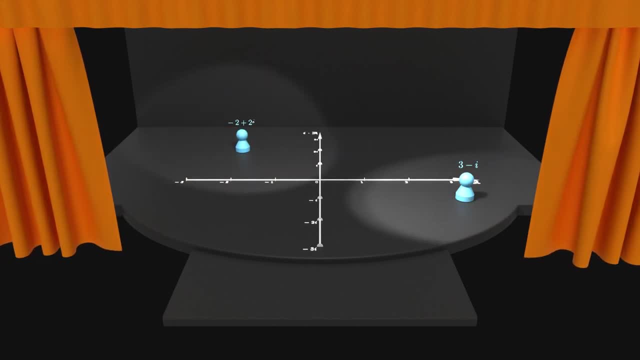 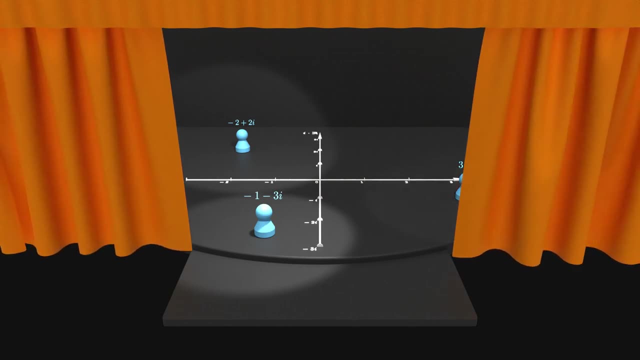 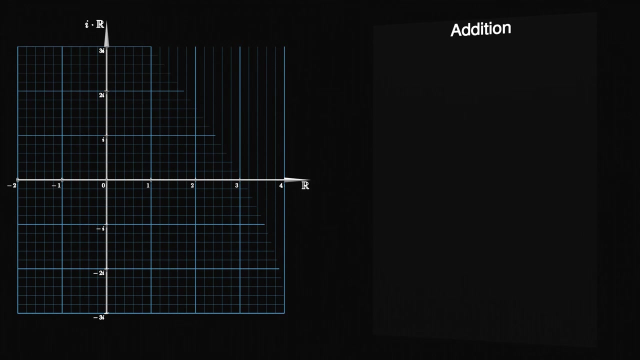 director writing the script. You need to tell everyone on stage where they have to be and how they have to move. Let's have a look at some stage directions you can give. Consider the complex numbers 3 minus i and minus 1 plus i. again The point associated. 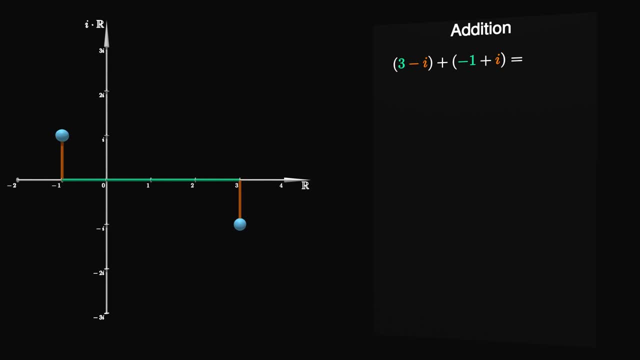 with their sum, can be found with the following four-step instruction: From the origin, move three units to the right, one unit down, one unit to the left and one unit up. As we already calculated, the result is indeed the complex number 2.. Notice how the first two steps just 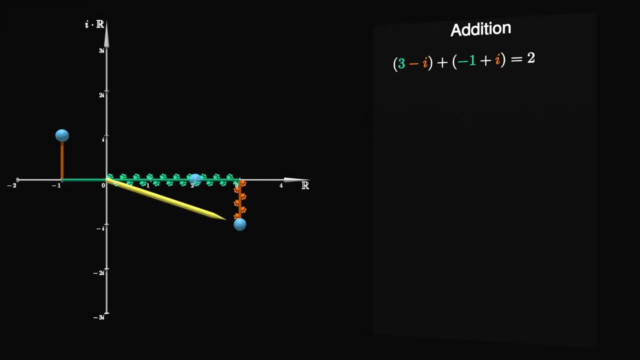 lead to the point 3 minus i. We could have taken a shortcut by drawing an arrow from the origin to this point. The last two steps can be simplified by drawing an arrow from the origin to minus 1 plus i and sliding its tail to the tip of the first arrow. Subtraction is just like addition. 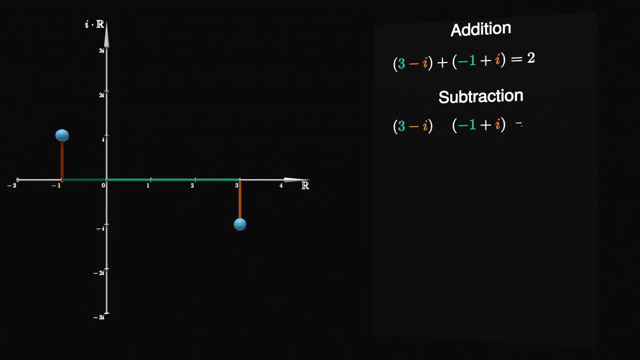 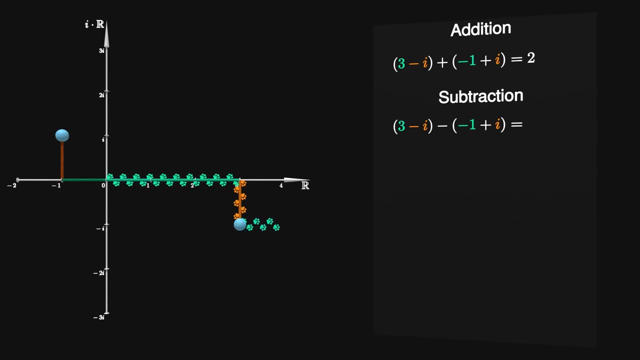 but the direction of the last two steps is inverted From the origin: move three units to the right, one unit down, but this time one unit to the right and one unit down. We can keep the first arrow. only the second arrow needs to be flipped to resemble the. 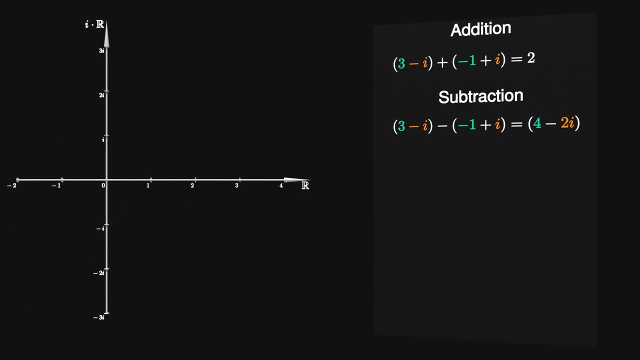 change of direction. Thinking of a complex number as a walking instruction or as an arrow makes it easier to visualize. Take 2 plus i as an example. Multiplying it with 2 corresponds with following the walking instruction twice, or, alternatively, with stretching the arrow to twice its length. 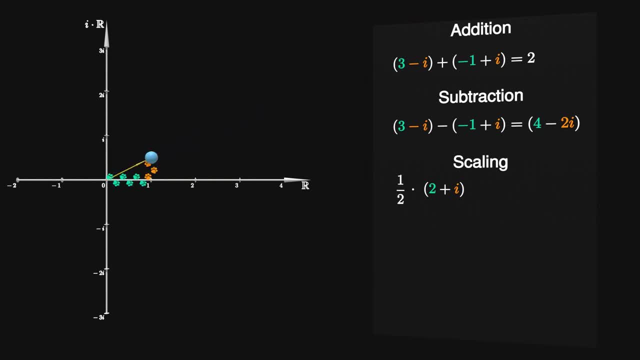 Conversely, multiplying with 1 over 2 squishes the arrow to half its length. A negative factor does the same, but also flips the arrow after stretching or squishing it. In general, we refer to this action as scaling. Notice how every point on the line going through 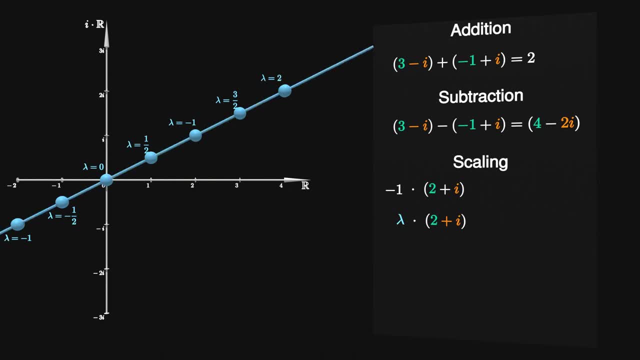 the origin and the complex number can be reached by scaling the complex number accordingly. Choosing a parameter lambda as the factor allows us to describe the action in the following way. We are now able to describe the unique line going through the origin and the given complex. 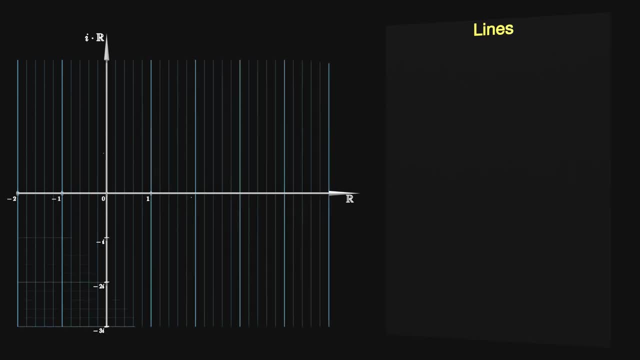 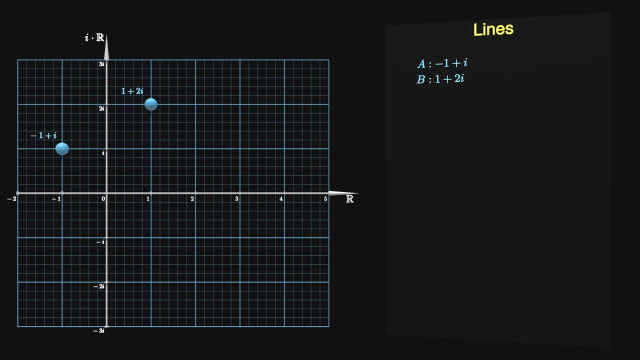 number. We can tweak this method in order to describe the line going through two general complex numbers. Take minus 1 plus i and 1 plus 2i as an example and notice that there is a unique line going through them. Choose one of the two complex numbers in this case. 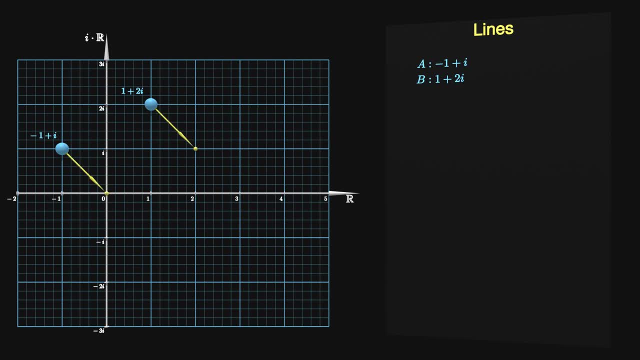 I chose minus 1 plus i and subtract the chosen complex number from the two original complex numbers. Here we get 0 and 2 plus i as a result. Notice how this shifts our two original complex numbers in a way that one of them becomes the origin. We can now describe the. 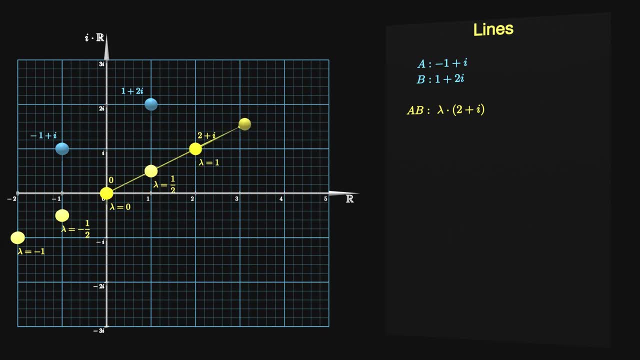 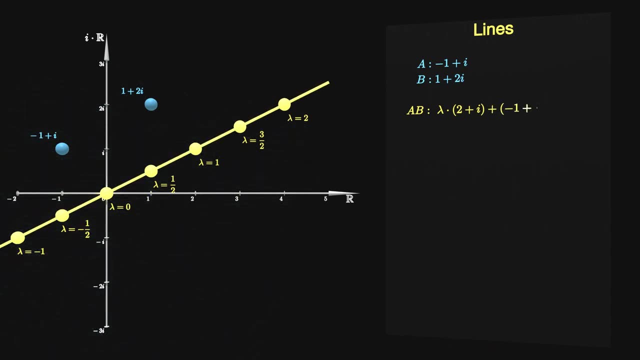 line going through them, in this case lambda times 2 plus i, but we need to shift this line to where it was by adding the subtracted value from before. This yields minus 1 plus i, plus lambda times 2 plus i. as a result, Of course, this expression can be tidied up. 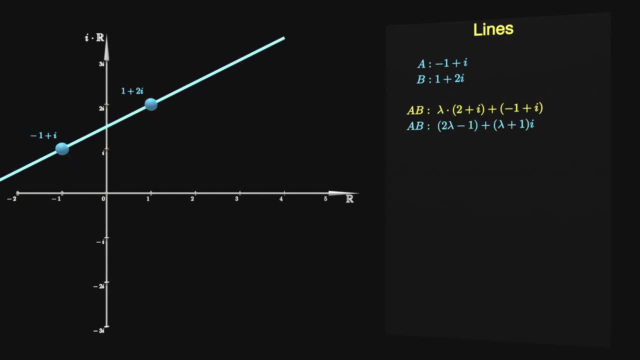 a little bit. This process can be done more quickly by condensing it into a single formula. Let z1 and z2 be two general complex numbers. The unique line going through them is described by the expression z1 plus lambda times z2 minus z1.. Consider the example: z1 equals 4 plus i and z2 equals. 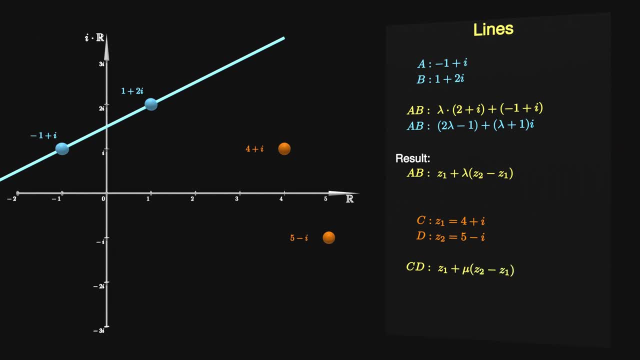 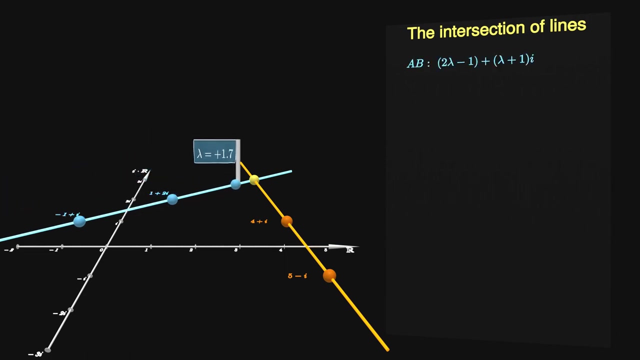 5 minus i. Since we already used lambda, we are going to use a different parameter, like mu, In order to distinguish both lines. We now gathered two expressions, with each of them describing a line in the complex plane. One interesting thing we can do with two different lines is to determine where they intersect. 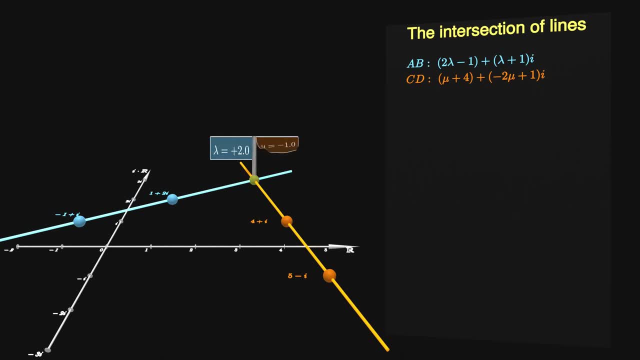 We do this by equating both expressions and solving the resulting equation. As of right now, we have one equation with two variables. However, notice that two complex numbers are equal if, and only if, their real parts and their imaginary parts are equal. The result is an easy to solve system of two linear equations. Plugging mu equals minus. 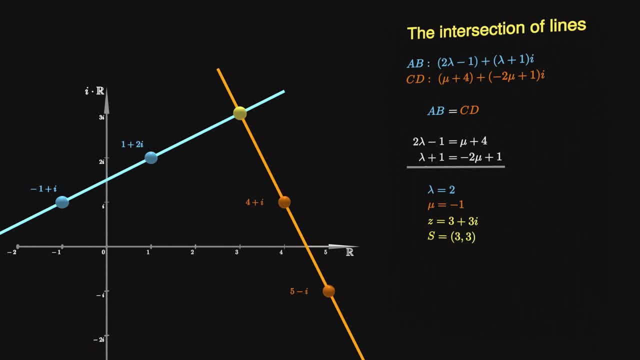 1 into the original line expression yields the point where the two lines intersect. We again need to determine what their local factors are. Again, the result turned out nicely just because I chose the example accordingly. Please don´t be scared if you encounter massive fractions while working out the intersection. 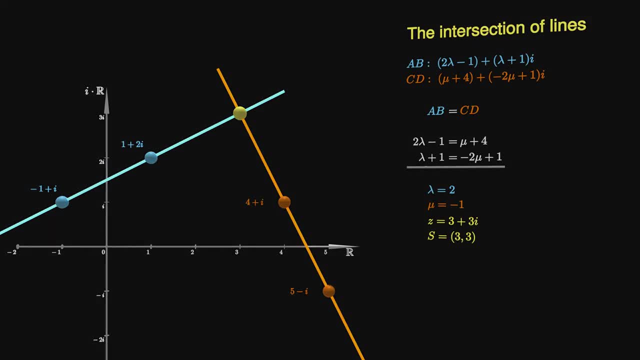 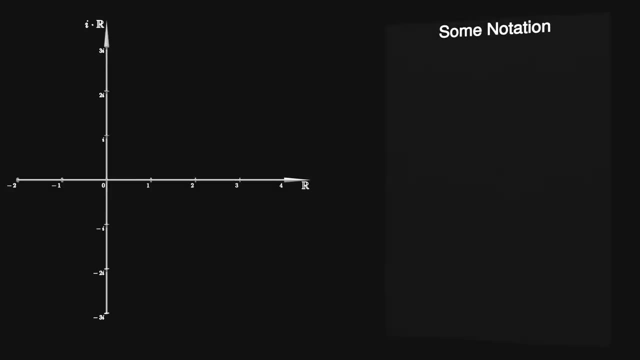 of two lines And keep in mind that there might not even be an intersection, since both lines could be parallel. In this case, the system of linear equations doesn´t admit a solution. We often times want to refer. We call this distance the absolute value of a plus bi, and we use this notation with two vertical lines. 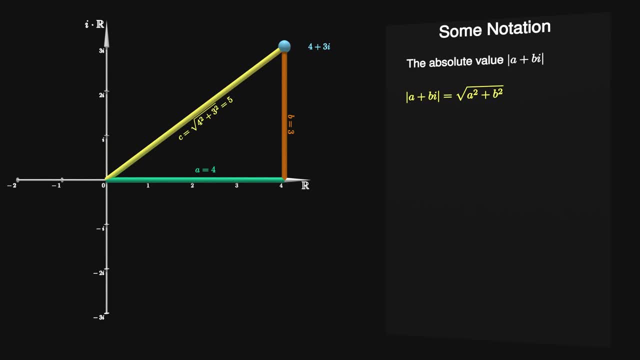 If we are only talking about real numbers, the absolute value can be understood as dropping any existent minus sign. When it comes to complex numbers, it can be calculated using the Pythagorean theorem. Now think of the angle between the real axis and the arrow described by a complex number: a plus bi. 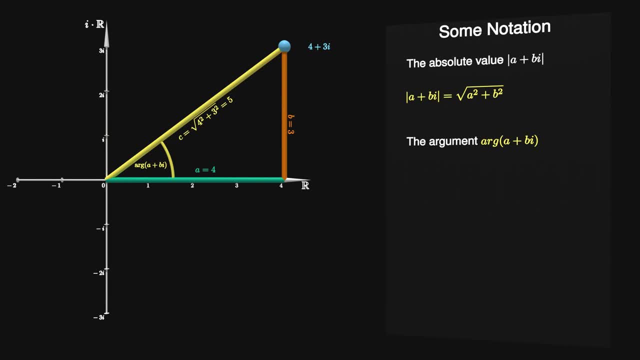 We refer to this angle as the argument of a plus bi and use the notation arc, a plus bi. where arc is short for argument, It can be calculated through the means of trigonometry, but this won't be necessary for this video. 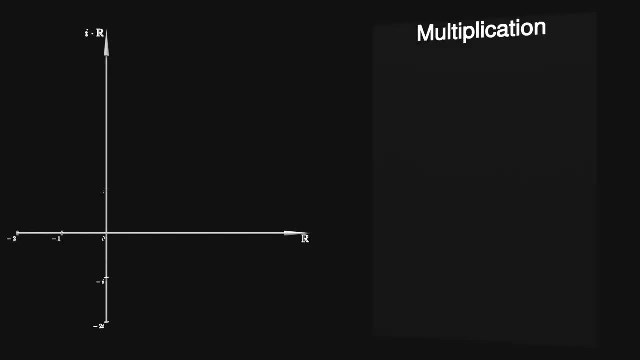 The astute scholars amongst you may have noticed that we only looked at linear algebra up to this point. This is certainly correct, But now comes the part where complex numbers outshine 2D vectors completely. Consider the complex numbers 3 minus i and minus 1 plus i again. 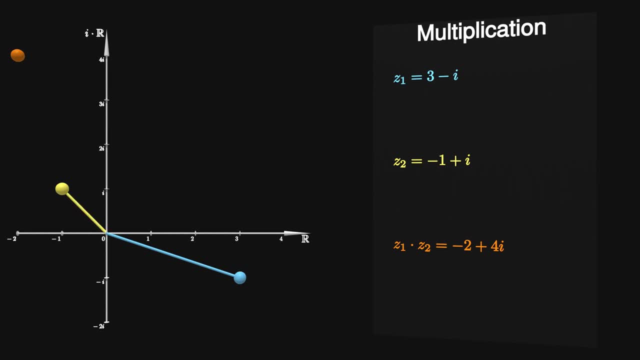 Their product can be derived as follows: First scale: 3 minus i by the absolute value of minus 1 plus i. Second, rotate the result counterclockwise around the origin by the argument of minus 1 plus i, The result of 3 minus i. 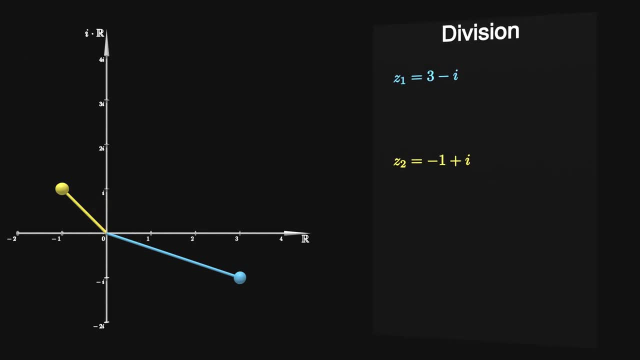 divided by minus 1 plus i can be derived in a similar way. First, scale 3 minus i by 1 over the absolute value of minus 1 plus i. Second, rotate the result clockwise around the origin by the argument of minus 1 plus i. 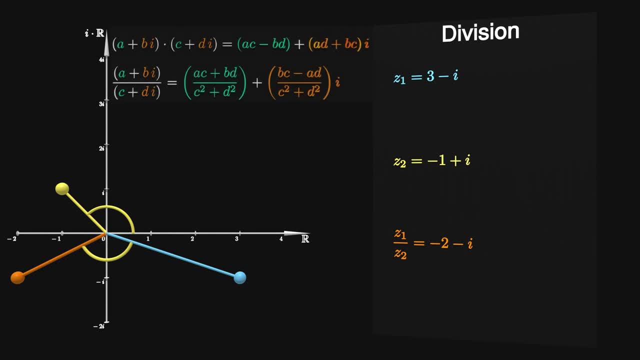 Of course, we already have two convenient formulas for actually calculating the product or the quotient of two complex numbers. The main takeaway here is that multiplication describes scaling and counterclockwise rotation around the origin, while division describes scaling and clockwise rotation around the origin. 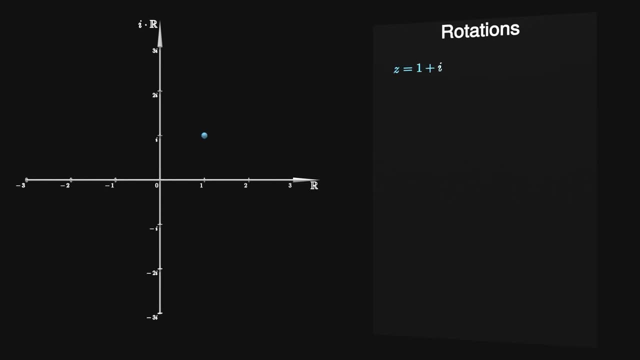 Let's consider the complex number 1 plus i. We want to rotate it counterclockwise around the origin by 90 degrees. Notice that the complex number i has 90 degrees as its argument. Additionally, the absolute value of i is 1.. 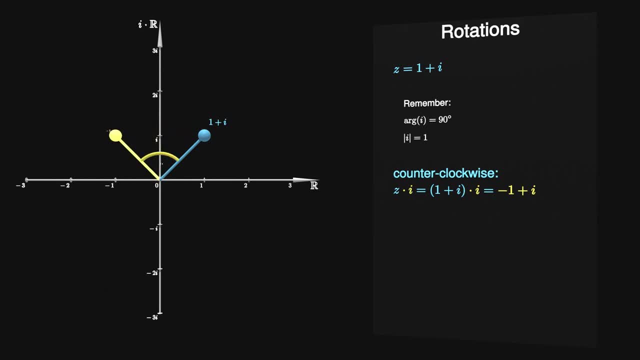 So notice that no scaling is going to occur while multiplying with i. We could have also rotated 1 plus i clockwise around the origin by dividing by i. But what if we wanted to rotate 1 plus i around another point, like 2i, for example? 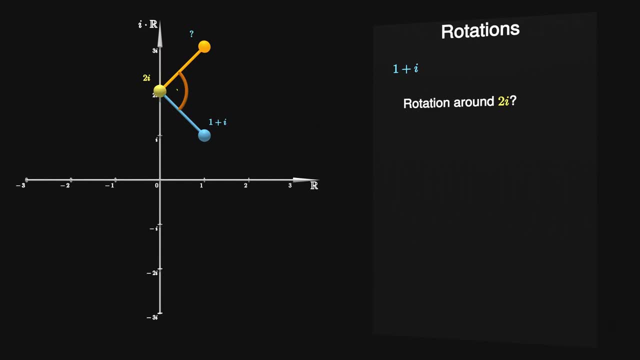 Let us see how this works. First, shift both points by subtracting 2i from them. from them, Notice how 2i was shifted to the origin. Second, multiply the result with i in order to rotate it counterclockwise around the origin by 90 degrees. Third, shift both. 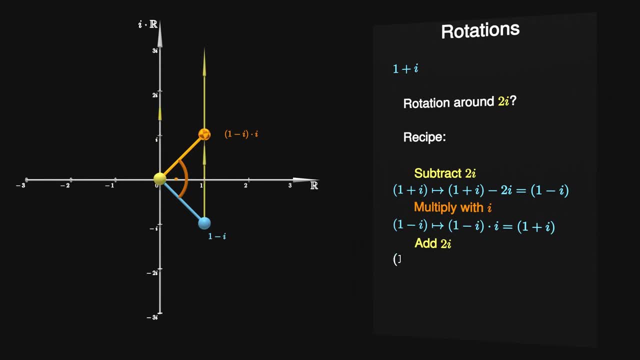 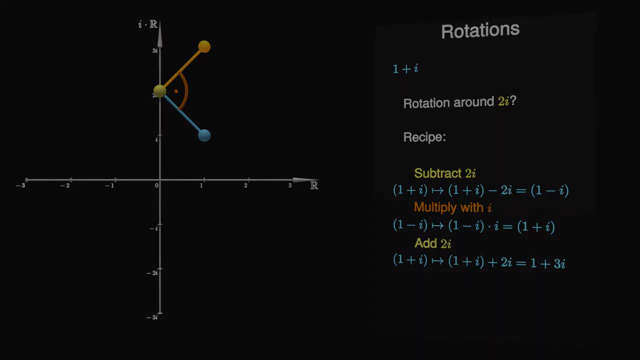 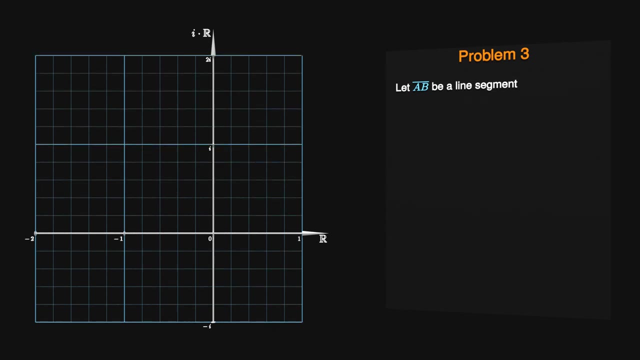 points back by adding 2i. This might seem surprising, but we now have everything we need to know in order to solve the geometry problem I presented at the start of this video. The problem starts out with the following proposition: Let a, b be a line segment, We. 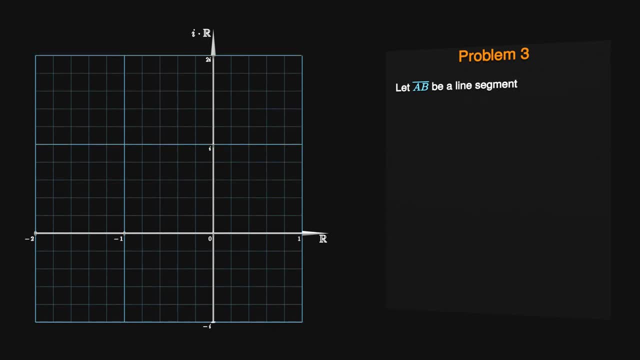 want the problem to take place in the complex plane, but where do we put a and b exactly? Some might suggest that we have to treat a and b as two general complex numbers, like a plus b i and c plus d i. This would work, but there is a way to make future calculations. 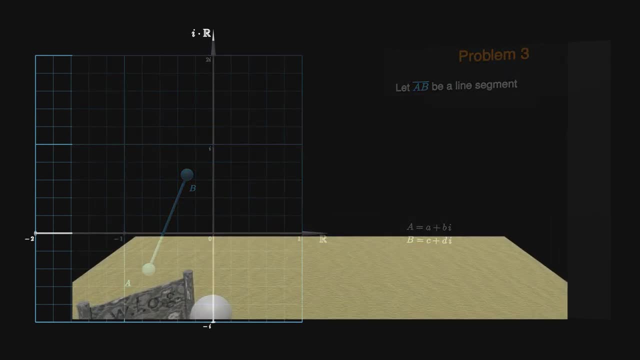 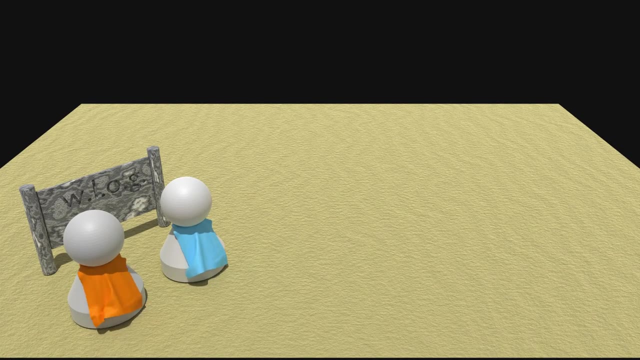 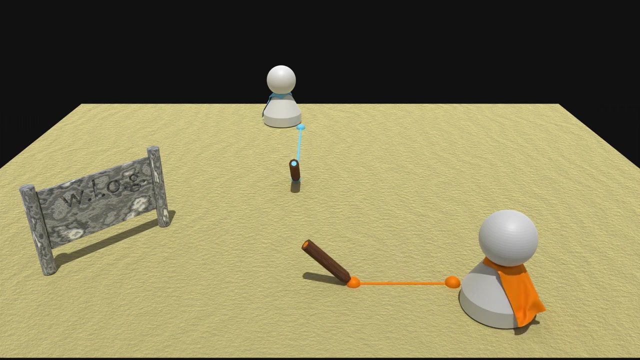 easier. Think of two ancient greek mathematicians sitting at the beach and studying GI Geometry by drawing figures in the sand. They are asked to imagine a line segment, and so they do by drawing one wherever they happen to sit. From there they follow the same unambiguous. 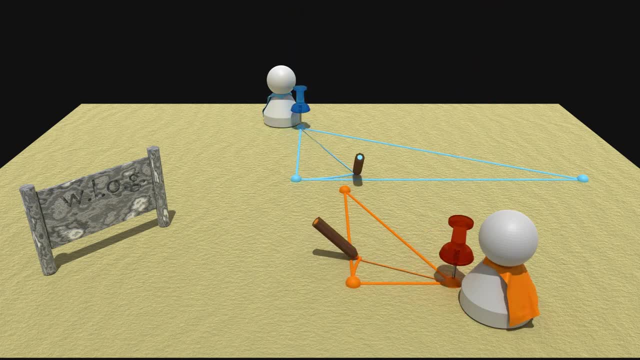 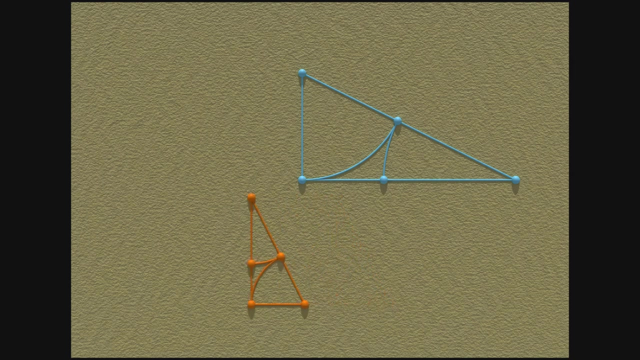 steps to produce some geometric construction. Both resulting figures are geometric. We can give the two corresponding limits for some of these equations, So we can draw one line segment and we can use a operations line segment to draw another line segment. This means that a and b are geometrically similar, meaning that we can scale, rotate. 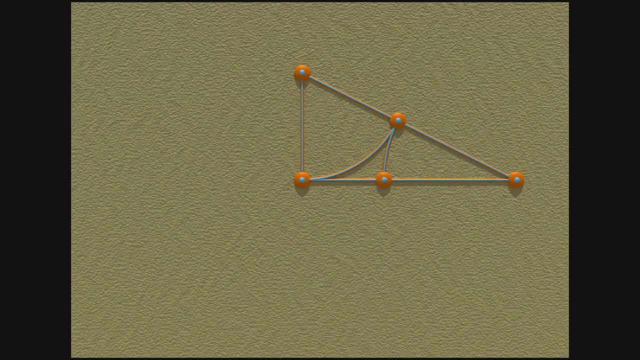 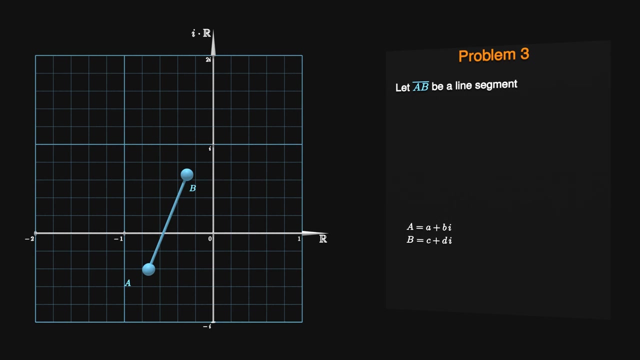 mirror and shift one figure in order to perfectly match the other. Consequently, it's sufficient to study just one figure, because any result is applicable to the other as well. Thanks to geometric similarity, we are free to choose a and b however we like, for example: 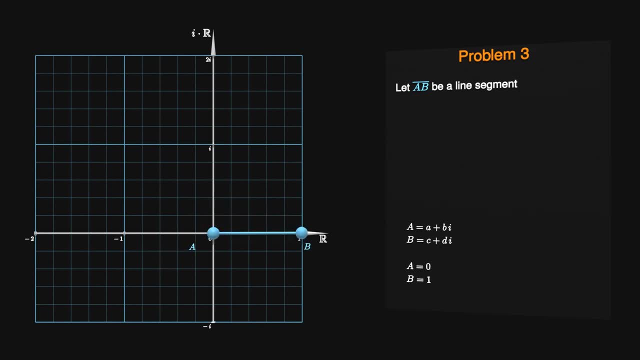 a equals zero and b equals one. The idea of showing this value is quite straightforward. If we want to determine the result, it's just taking a and d. but if we want to use a and b, then we know how to perform them. 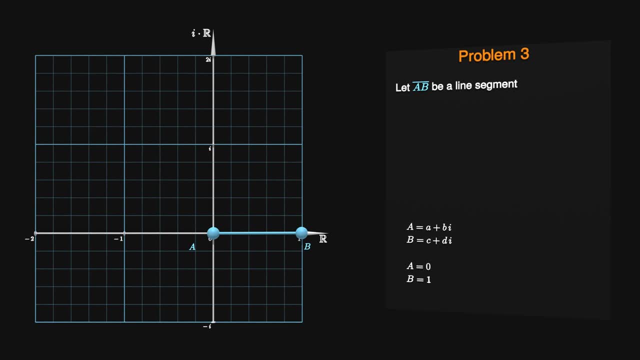 So let's look at the three order equation. focusing on a special case that is geometrically similar to the general case can be referred to with the expression without loss of generality. For example, mathematicians would distill everything we talked about in this section. 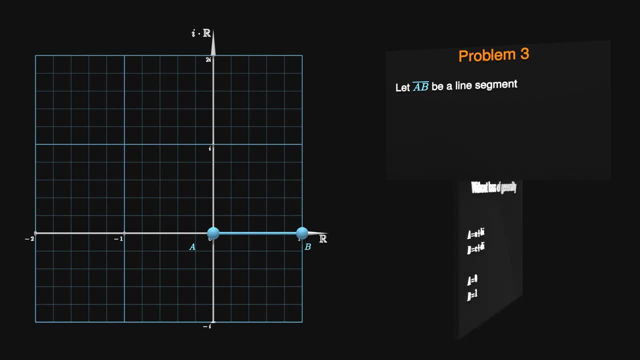 down to the following sentence: a equals zero and b equals one is assumed without loss of generality. The geometry problem now asks us to imagine a point t on the line segment that is closer to b than to a. Now you might be thinking that we are free to choose t, just like we were free to choose. 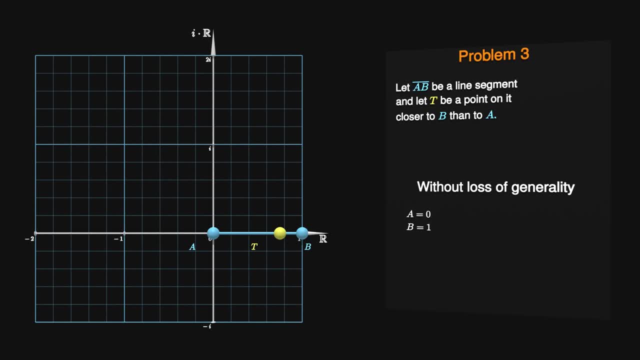 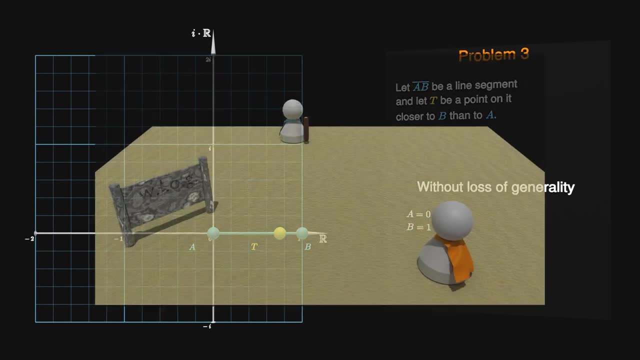 a and b. Unfortunately, it does not work this way because the instruction closer to b than to a is ambiguous. Imagine the ancient greek mathematicians again, If one of them chose t to be near the middle of the line segment and the other one chose 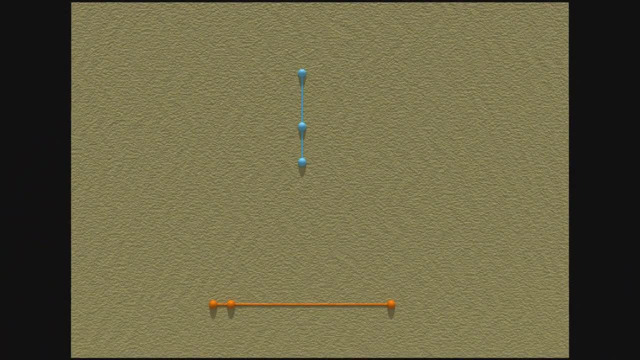 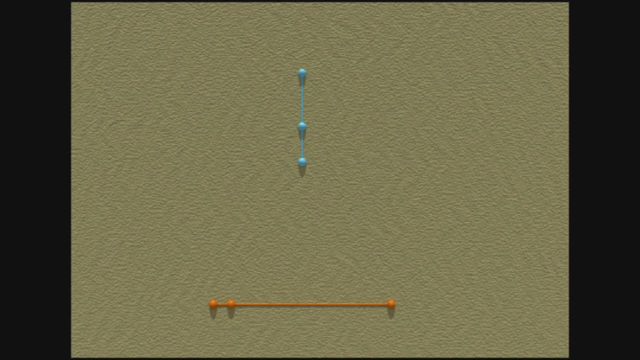 t to be near the point b, they would end up with figures which are not geometrically similar. In fact, they don´t need to be close to the line segment, because the point b is closer to b than to a to draw the whole figure. for this to be seen, Focus on the line segment AB with t on it. 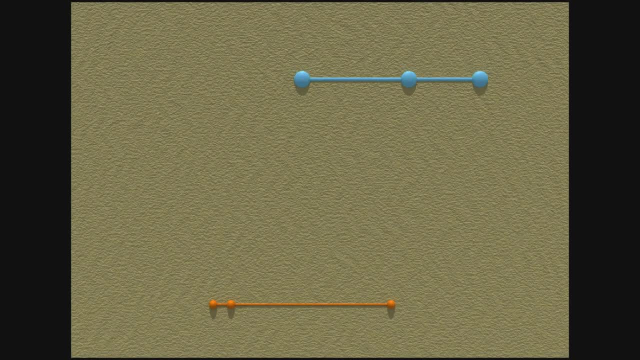 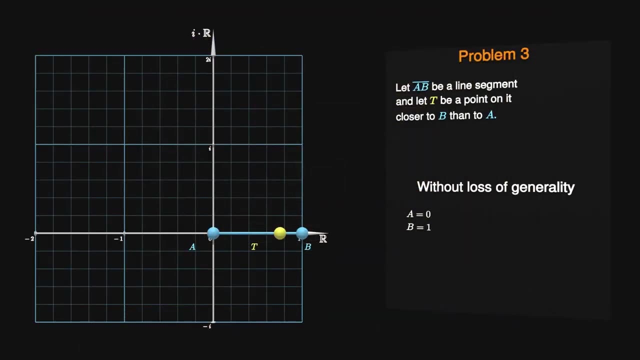 There is no way to match them by scaling, rotating, mirroring or shifting them. For this reason, we need to treat t as a general point. We do this by making use of the parameter t equals x, where x is a real number in the semi-open interval from 0.5 to 1.. 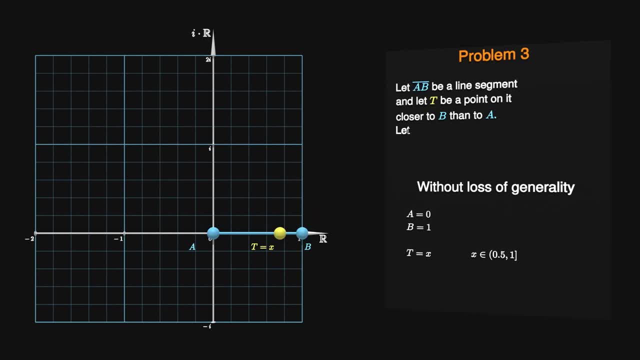 Now the problem asks us to imagine a point C on the line that is perpendicular to AB and that goes through t. Just like with t, we need to treat C as a general point. but notice that we can assume C to be above the line segment without loss of generality. 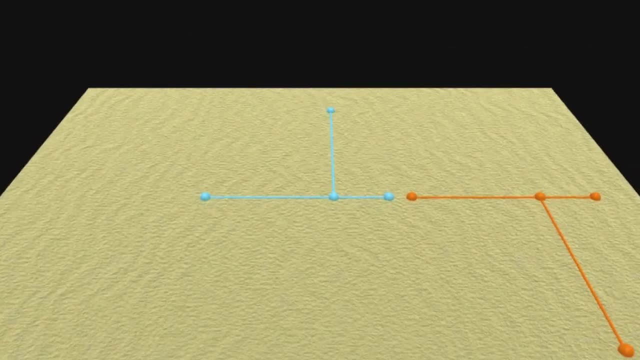 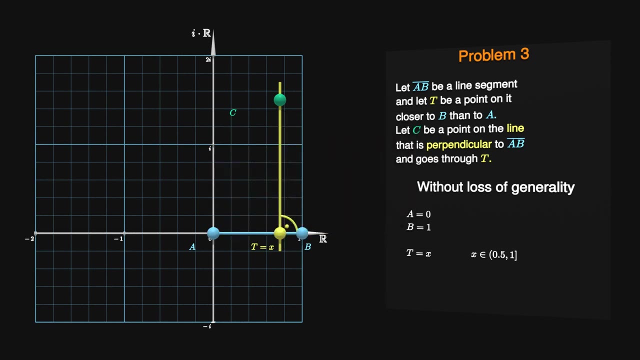 If C were to be below it, we could just look at the drawing mirrored along the real axis and end up with a geometrically similar drawing where C happens to be above the line segment. We can therefore assume C equals x plus yi without loss of generality. 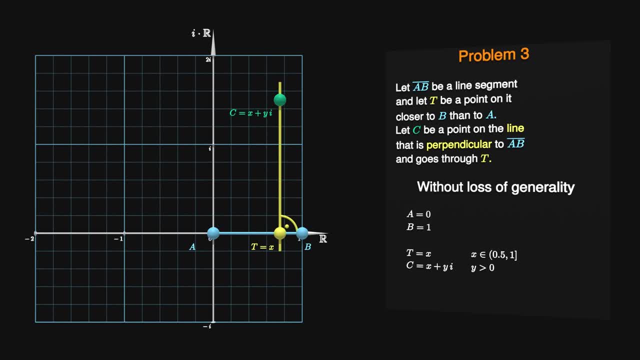 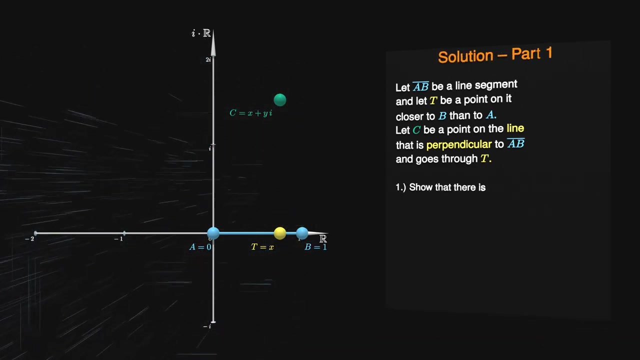 where y is a real number bigger than 0.. Abusing geometric similarity in order to make simplifying assumptions acts as the concrete foundation for our mathematical proof, because it fixes many moving parts. We can now start to dig into the main calculations. We first have to show that there exists exactly one point D on the line segment AC. 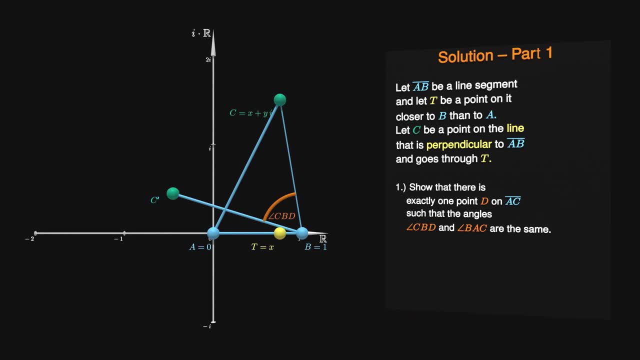 such that the angles CBD and BAC are the same. Here's how we are going to do that. First, rotate C counterclockwise around B by the angle BAC and call the result C' Second, find the intersection of the line going through B. 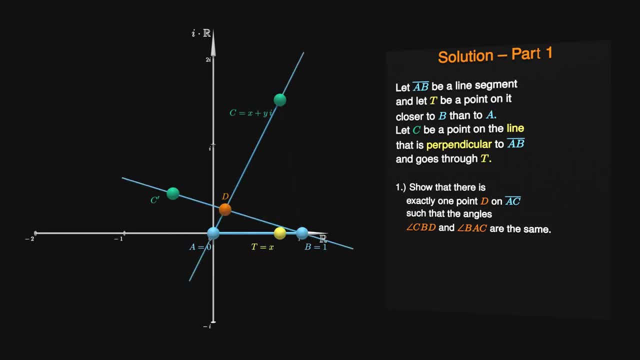 and C' with the line going through A and C. This intersection is the point D the problem was talking about At the end. check if D lies on the line segment AC. Notice that C itself has the argument of the angle BAC. so let's start with the rotation. 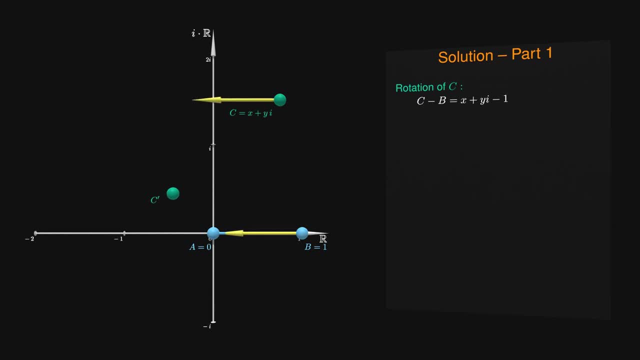 Subtract B from the points B and C. This shifts B to the origin and C to the point x-1 plus yi. Now multiply this result with C in order to rotate it counterclockwise around the origin by the angle of BAC. Some scaling occurs as well. 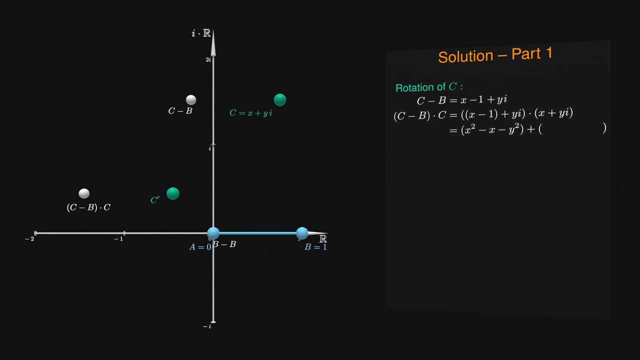 but this effect doesn't matter, for reasons that are going to become apparent. Finally, rotate B to the origin and C to the point x-1 plus yi. Finally, we need to shift the result back by adding B to it. We have finally found an expression for C' but we only care about the line going through B. 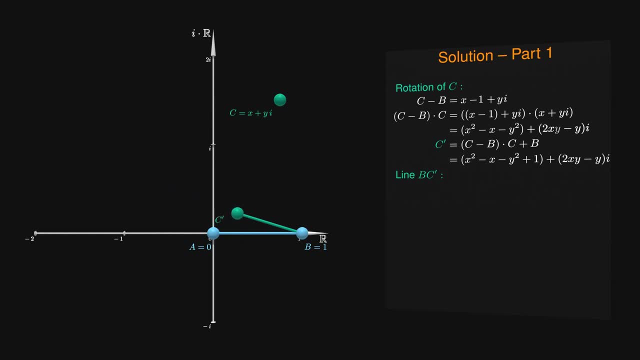 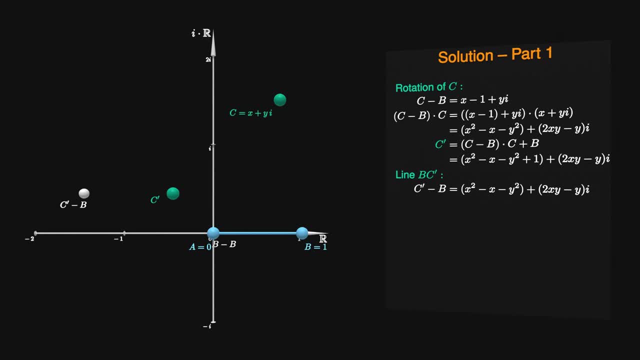 Subtract B from the points B and C' Subtract B from the points B and C' This again shifts B to the origin and C' to the following point. Second, multiply it by the parameter lambda to describe the line And finally shift the result back by adding B to it. 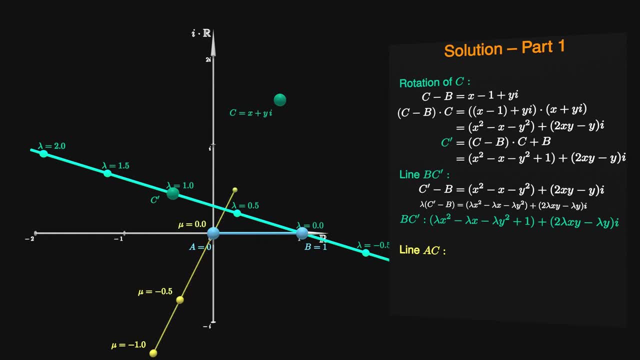 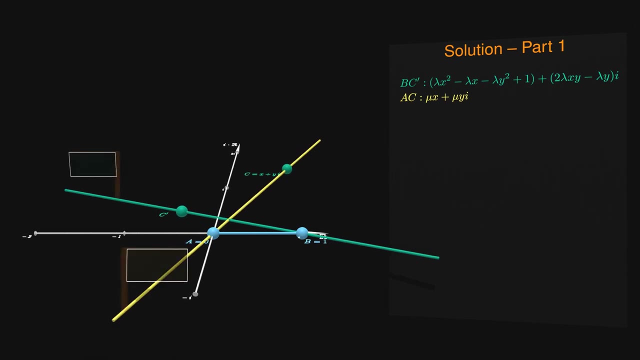 The line going through A and C is easier to describe, since A is already at the origin. We just need to scale C by a parameter like mu. Equating both expressions leads to the following system of linear equations: We need to figure out the values of the parameters mu and lambda. 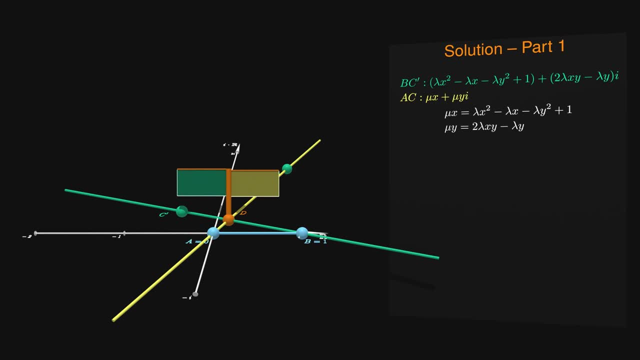 in order to get the point where both lines intersect. Since y is bigger than zero, we can divide the second equation by it. Mu can now be eliminated in the first equation by replacing it with 2 lambda, x minus lambda, We have solved for lambda and we can use this result to solve for mu as well. 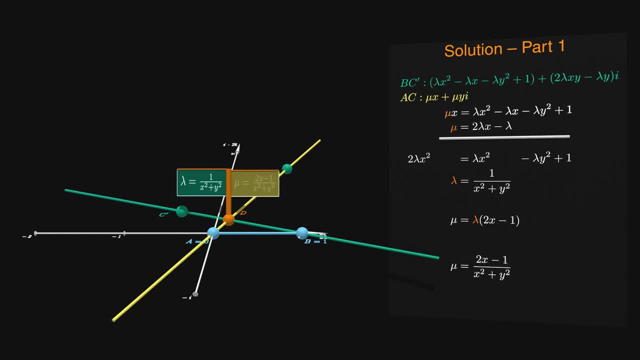 You could go ahead and calculate the point D, but we can already tell that D is greater than zero. This check is done by looking at the value of the index, value of the second bottom line. Let's say d is greater than zero, We must estimate d plus a. 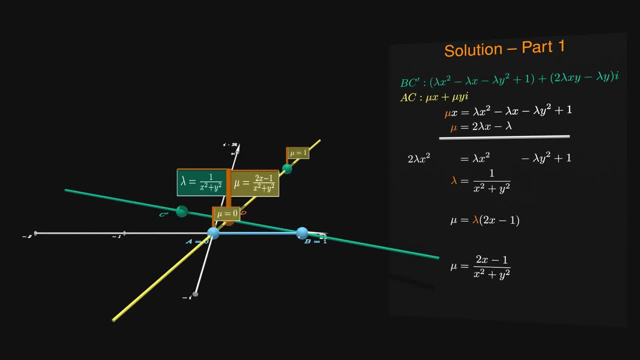 We can compare this with the value of the second line, which is greater than zero. Here we can see that the denominator 2x minus 1 lies on the line segment AC by just looking at the calculated value for the parameter mu. If we can prove that this value is between 0 and 1, then D has to be between A and C. 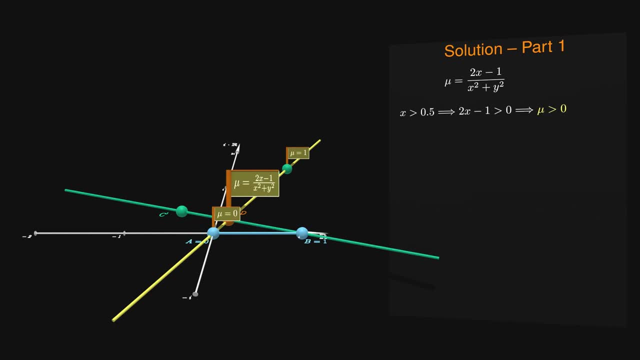 Since x is bigger than 0.5, it bigger than zero as well. We are left to show that this fraction is not bigger than one, and there's a pretty cool trick to do that. Consider x minus one: squared, It is the square. 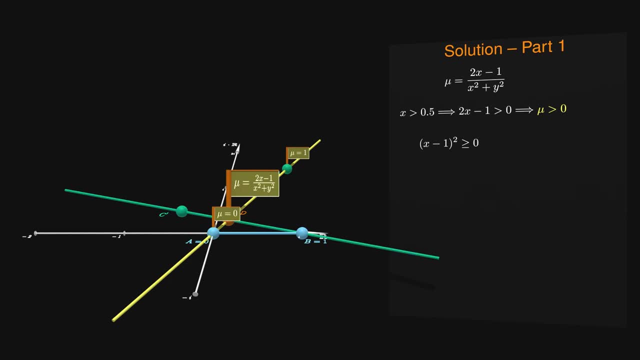 of some real number. therefore it's not negative From here. it's just simplification. The fraction two x minus one divided by x squared is not bigger than one. but it is even smaller if y squared is added to the denominator. The system of linear equations has exactly one. 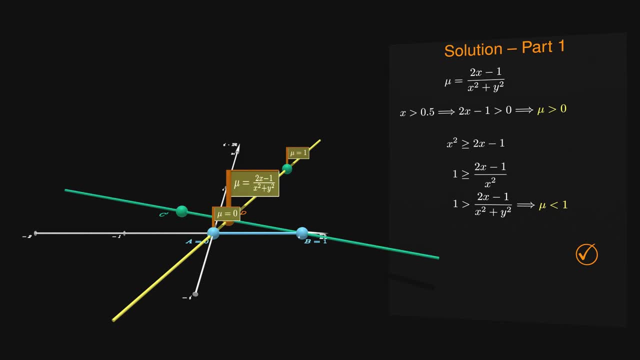 solution for the values of lambda and mu. Also, we have shown that the value of mu is always between zero and one. Therefore, there is exactly one point d between a and c, such that the angles cbd and bac are the same. We have solved the first part of the problem. Let's move on to the second. 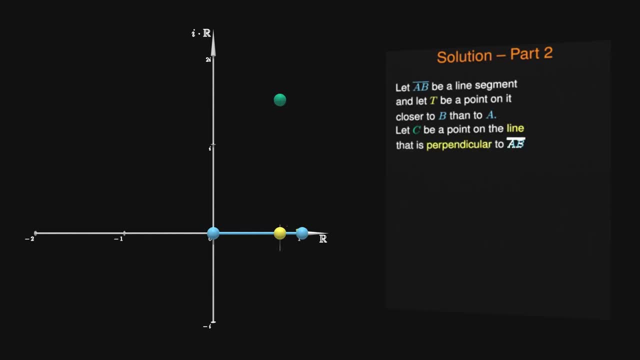 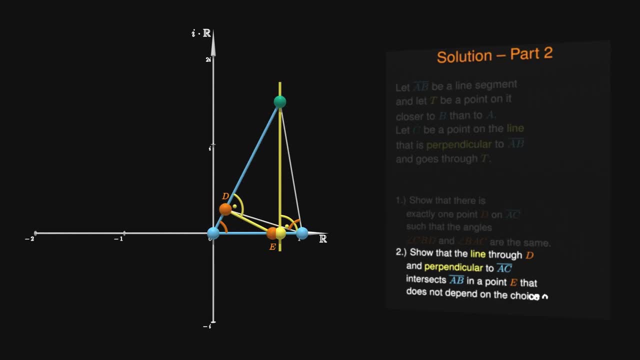 in a point e that does not depend on the choice of c. This part of the problem is going to be solved in the exact same way As of right now. we just know that d is somewhere on the line segment ab, but we need to calculate its exact position. 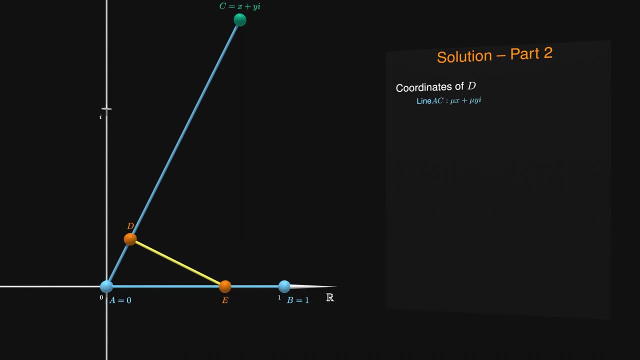 We do this by simply plugging in the calculated value for a parameter into the corresponding line expression. Take mu, for example. Next, we need to describe the line perpendicular to ac and going through d. We can get this line's expression by rotating a around d by 90 degrees and calling the result a prime. 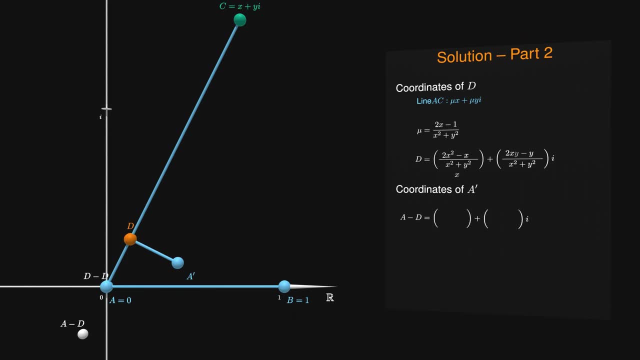 Subtract d from the points a and d. This shifts d to the origin and a to the following point. Multiply the result by the imaginary number i. This corresponds with a counterclockwise rotation around the origin by 90 degrees. Shift the result back by adding d to it. We have now obtained a prime Again. 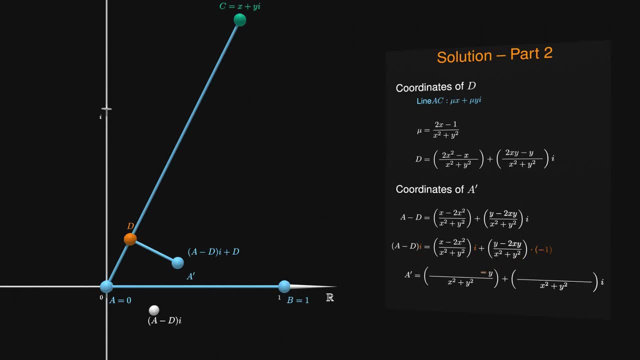 any scaling during multiplication doesn't affect the line. But notice that the imaginary number i has the absolute value 1.. In this particular case there was in fact no scaling. Now comes the part where we calculate the line expression for d: a prime Subtract d from d and a prime. This shifts d to the origin and a prime to the following point. 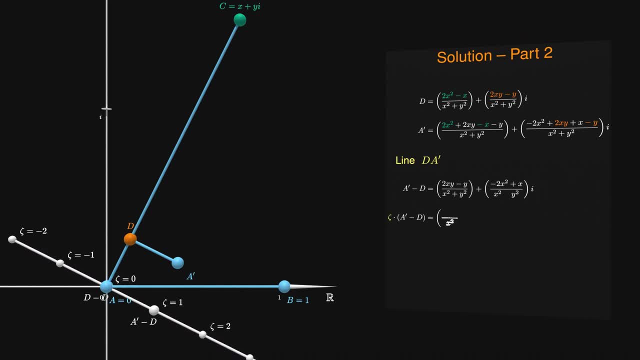 Now we can get the line expression. Multiply this result by a parameter like zeta. Add d back to this expression to shift the line accordingly. Please don't get intimidated by this line expression. We just need to know where this line intersects the real axis in order to obtain the point e. We do this by equating. 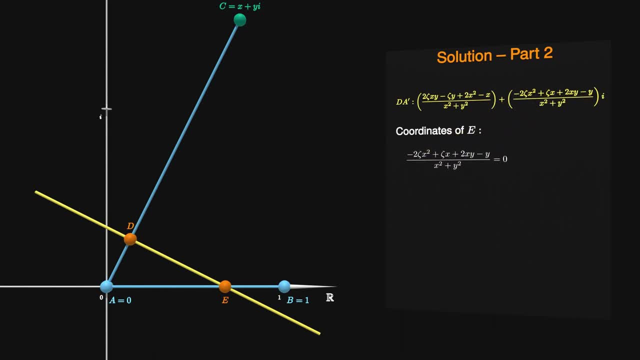 the imaginary part of the line expression. with zero and subtracting the imaginary number e, solving for Zeta, The line dA prime meets the real axis where Zeta equals the fraction we just obtained. but it can be simplified further. What a nice result. Now let's plug this value into the original line expression. 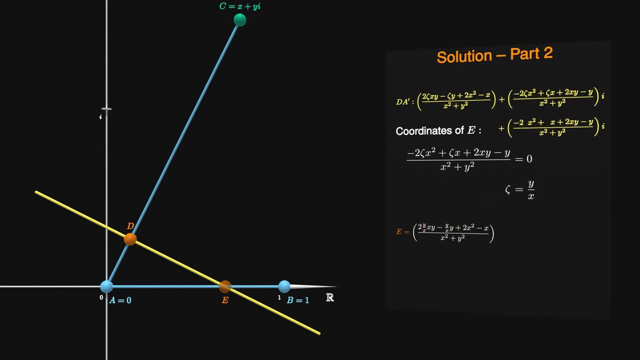 of dA prime in order to obtain E. Try to appreciate how everything works out perfectly in this calculation. Look at the expression for the point E and notice the absence of the symbol Y. This proves that E is indeed independent of the choice of Y, No matter how we choose C, the point E. 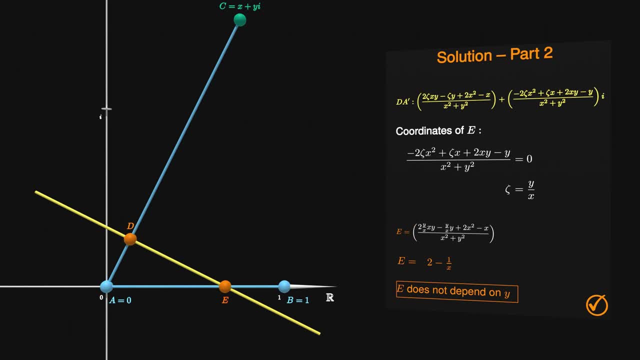 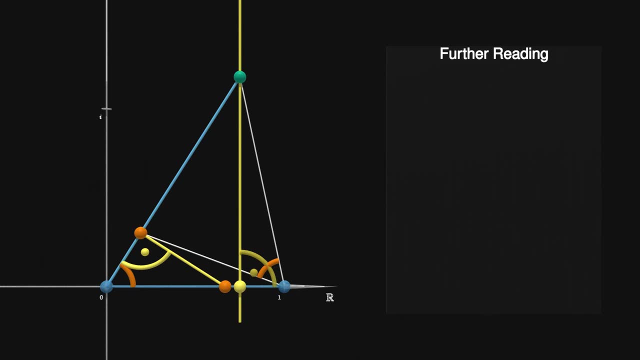 stays at this exact spot, And this is what the problem wanted us to prove. This video is an effort to make higher level mathematics more accessible to school students. You can find the proof I just presented in the video description. Feel free to use it as a template for your own proofs If you're interested in. 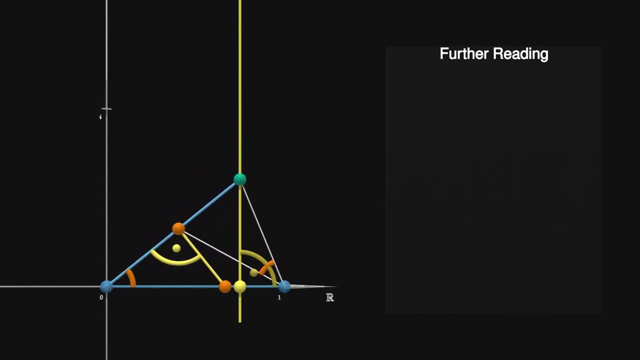 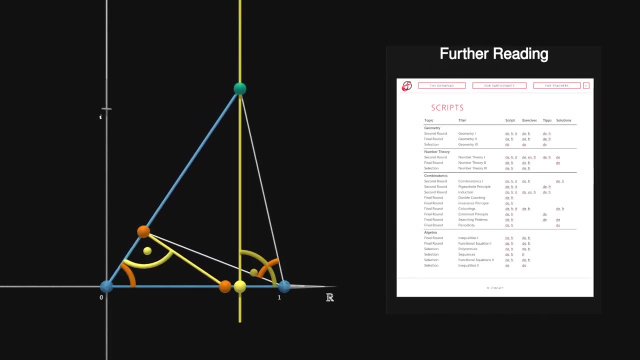 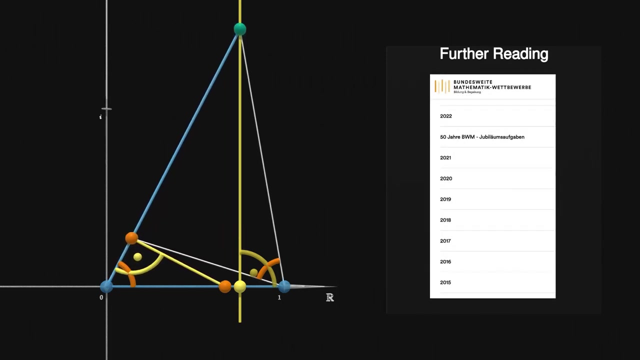 preparing for a math Olympiad and if you happen to speak German, French or Italian, I highly encourage you to study the free online resources provided by the Swiss Math Olympiad. The link can be found in the video description If you are interested in an elementary solution to the discussed geometry problem. 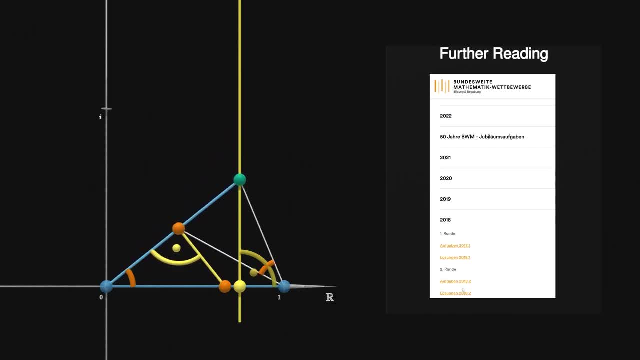 and if you happen to speak German, you can check out the official homepage of the Bundeswettbewerb Mathematik. There you can find further information about this math competition, as well as past problems with solutions. Again, the link can be found in the video description. Thanks for watching.